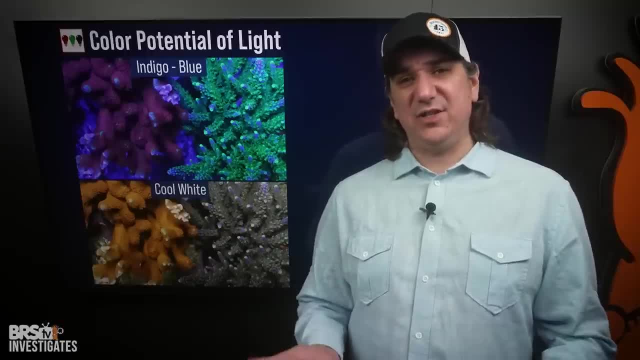 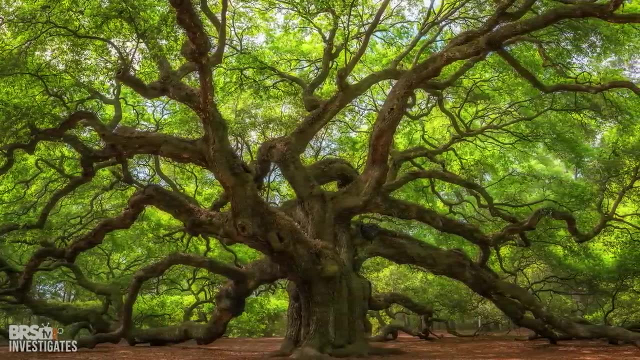 example of color pigments is how the sun makes most leaves look green. This is simply because the leaf is absorbing most of the sun's light for photosynthesis, but contains a color pigment that reflects green off its surface and back at your eye, and that's why it looks green. 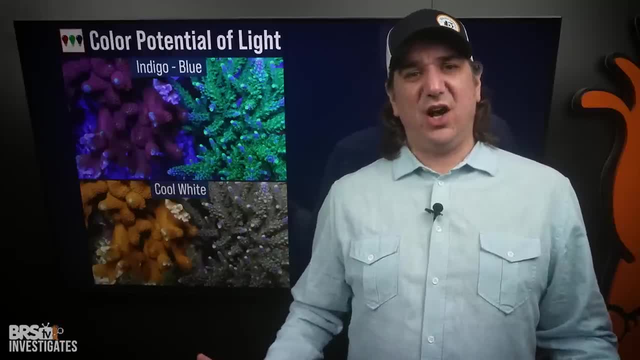 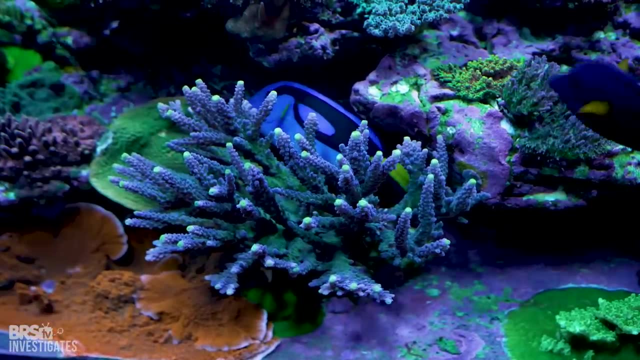 This effect is the same with corals. The reason that many corals have a certain color is simply because your light has that color and they are reflecting that color back at your eye. This is particularly true with purple and blue corals. They look like that shade because the 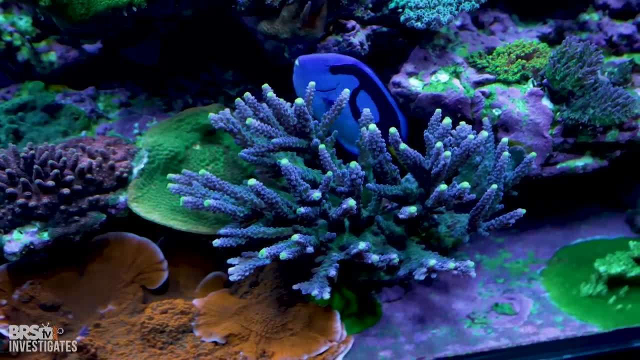 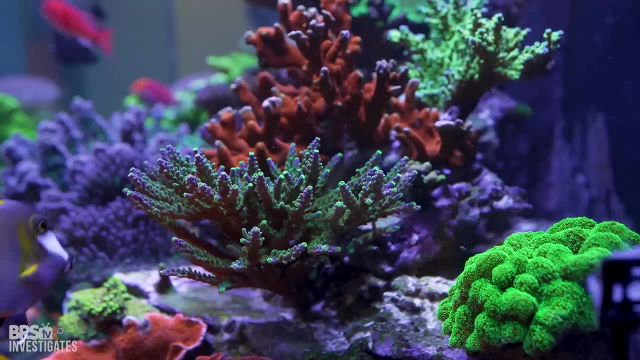 coral contains a violet to blue color pigment that is being reflected back at your eye. The second source of color, and probably the most desirable, is called fluorescence. Fluorescence is when the coral takes in high energy blue light and then re-emits it back out. 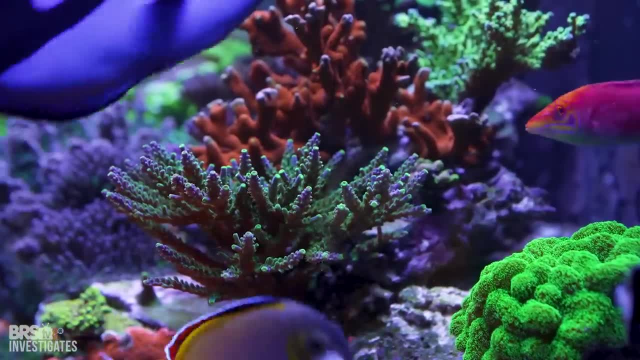 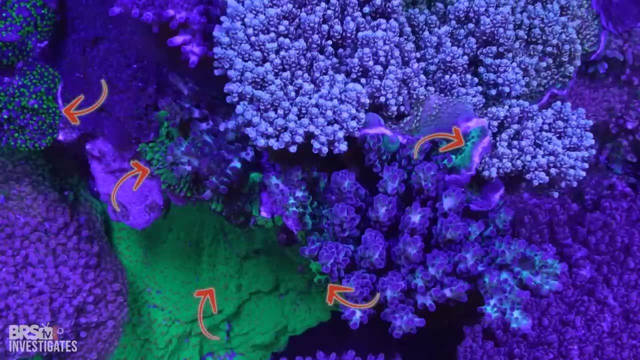 as a lower wavelength color like green, yellow, orange or red. If you want to know which corals have fluorescence in your tank, that's simple: Turn on only the blue lights, and anything that's not blue contains fluorescent proteins, The reason why reefers are often 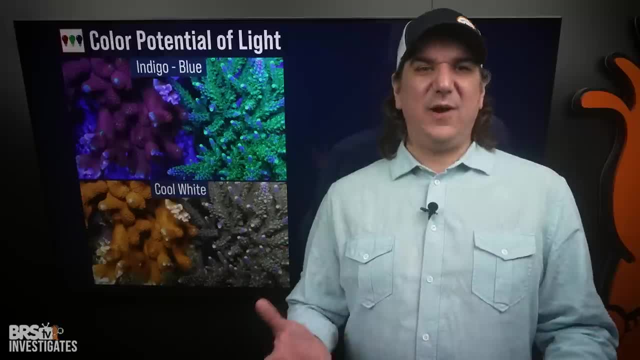 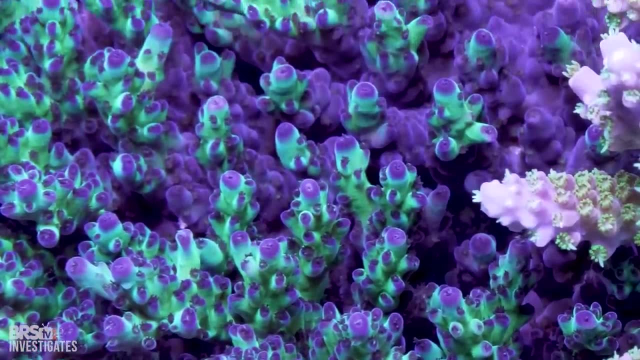 chasing fluorescent proteins over color pigments is. fluorescence isn't just a change of color, it's a glow that creates a very contrasty color pop and visually stunning display. The third source of color is an illusion. Many corals that are purple are not purple pigments. 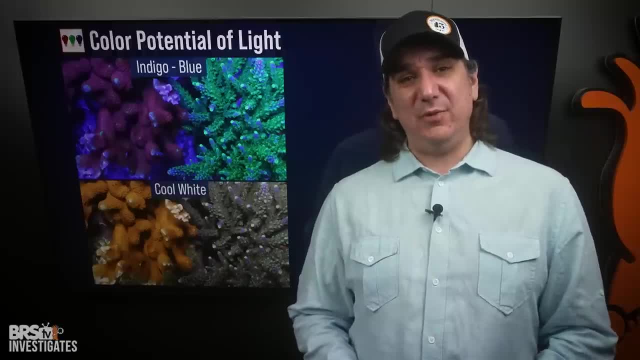 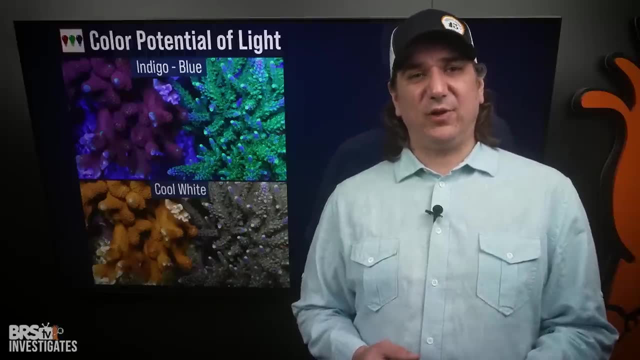 actually just a blend of blue and red pigments that, when illuminated with blue and red light, blend together to create purple. This is true of fluorescence as well. blue light and red fluorescence make purple too. In fact, most of the colors that you see in your 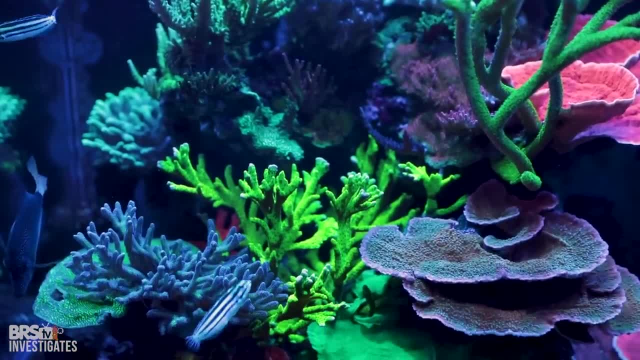 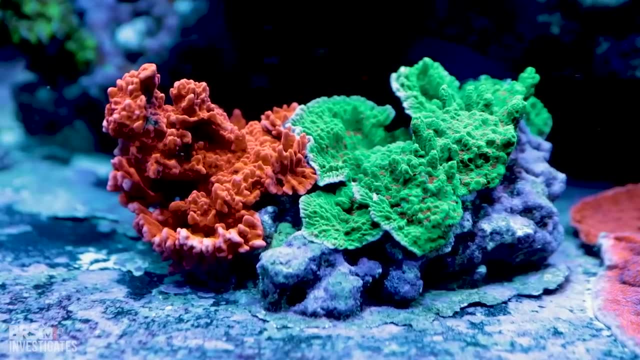 corals are just an illusionary effect of a blend of a multitude of color pigments and fluorescence, and then the light spectrums combined together to create the color that we perceive. With color pigments, fluorescent proteins and blending in mind, let's get to the test. 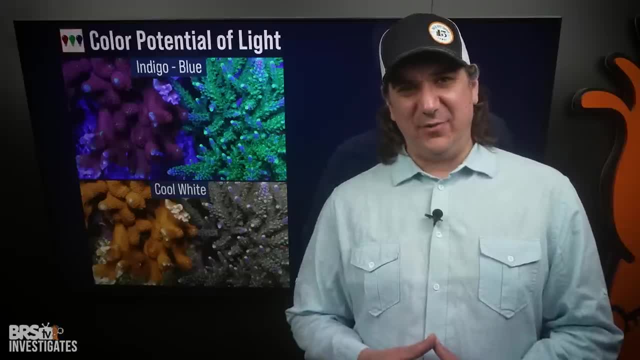 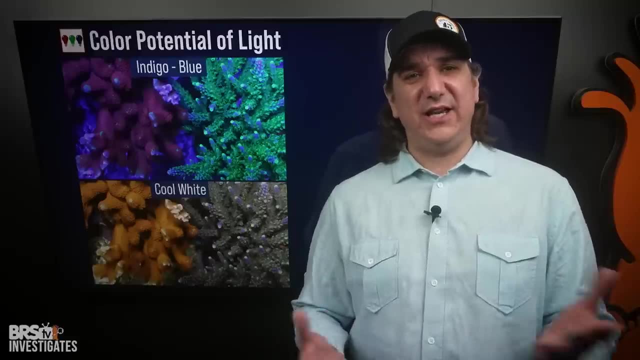 First, out of corals we selected to demonstrate how the deeper violet range, typically referred to as a tinnic light, highlights many corals natural fluorescence differently than the low energy indigo blue and light blue. We're looking for how specific shades of violet and blue can. 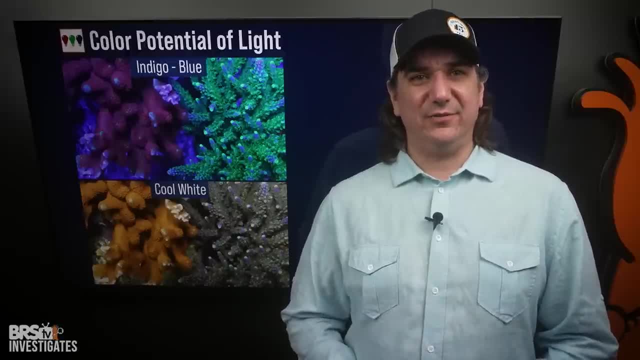 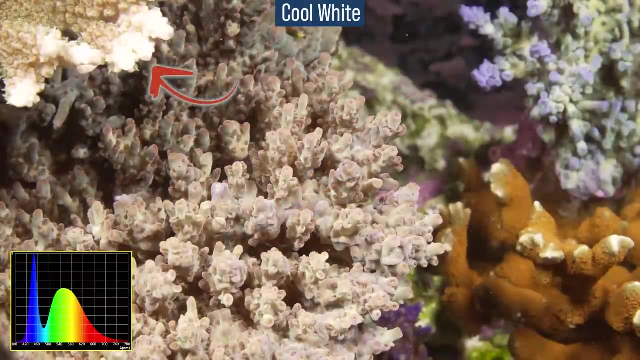 turn into that natural fluorescent glow that most reefers are after Under white light. the primary coral in this example is a drab washed out green, but note the brownish orange neighbor, as well as the white growth tips above it. White is the balance of all colors, so you'll see the 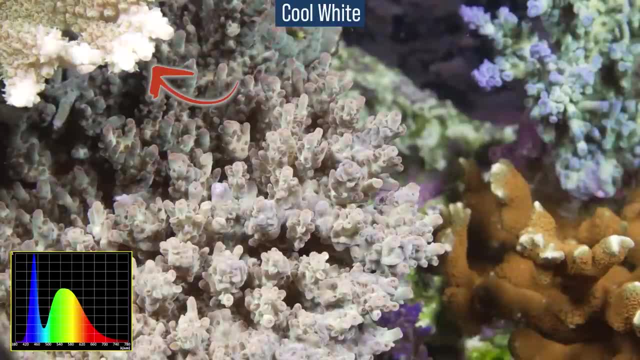 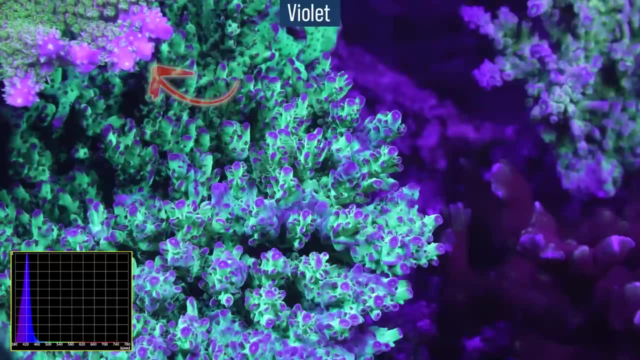 individual spectrums noted in those growth tips, which is a great reference against fluorescence. Switching to violet, you can see the violet light being reflected back at the eye on those white tips. This is essentially the color of this light. The rest of the coral tissue is now absorbing that. 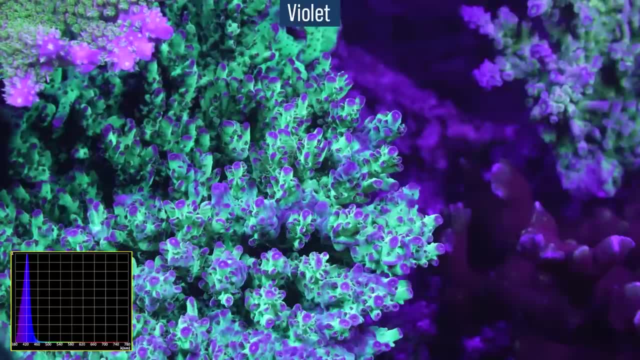 violet light and then re-emitting it back out as lower energy green. Note that it would appear that about 80 percent of the coral's tissue is fluorescing and that that orange brown coral on the right is still drab, Switching to indigo blue. an interesting effect happens here. 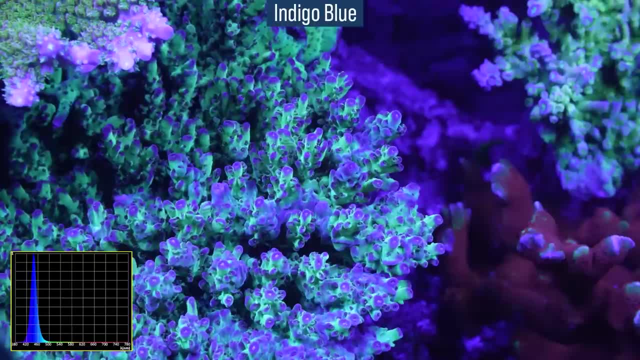 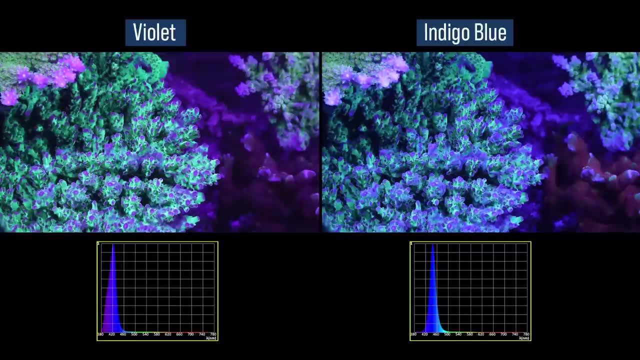 The tissue clearly has more of this bluer pigment in it, which can be seen in how the coral is now about 50 percent fluorescence and about 50 percent that purpley blue pigment. Side by side you can see how the violet light is weighted to highlighting the fluorescence. 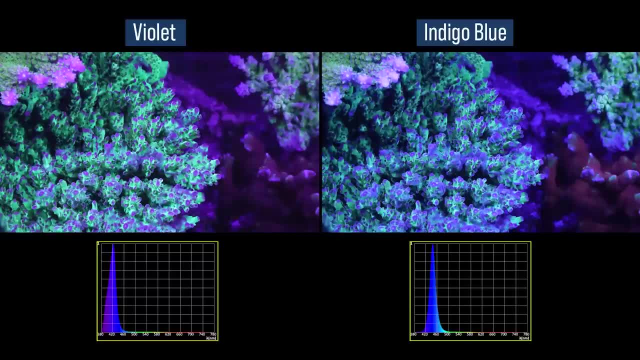 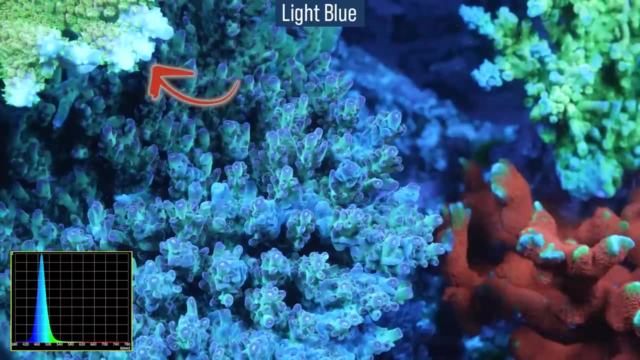 over color pigments and the brown coral is starting to see the orange fluorescence come out. Light blue continues these trends. The coral tips are now clearly reflecting light blue light. The light is now highlighting maybe 25 percent fluorescence and 75 percent light blue color. 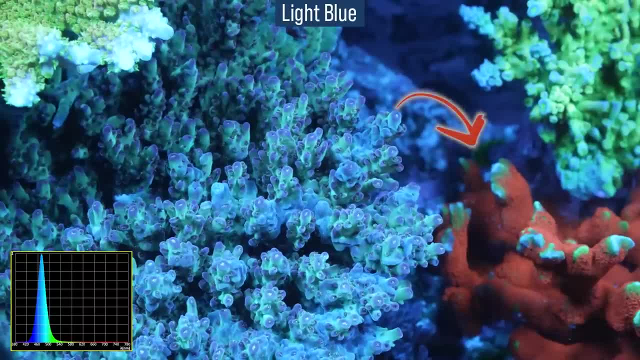 pigments, Most notably the brown coral, is now popping orange fluorescence and light blue pigments. The biggest takeaway here is that a spectrum of light, blue and orange fluorescence that makes one coral look drab might be the exact same spectrum that highlights another coral, the 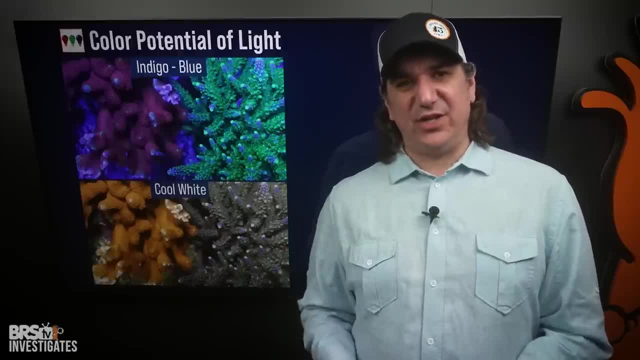 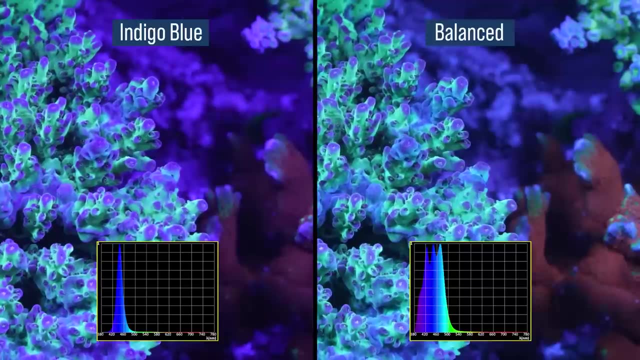 best. So the question is: can you combine them all together to capture the best of them all? and the answer is yes. In this case we balance the peaks almost equally. On the left is just a thin blue peak of indigo blue alone which fluoresces. great, but kind of one note. On the right, 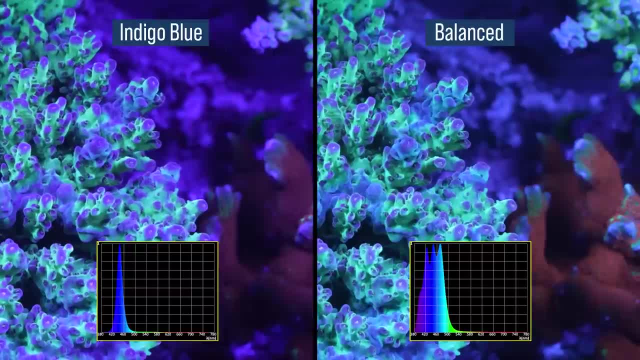 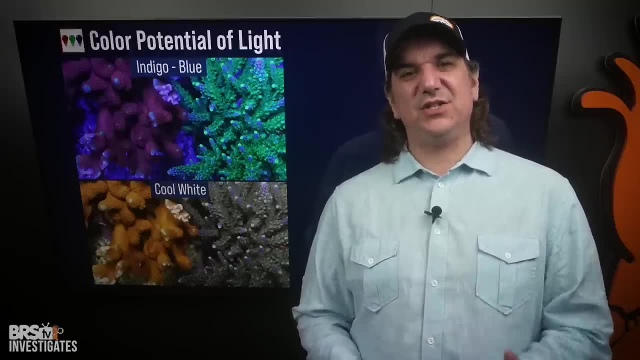 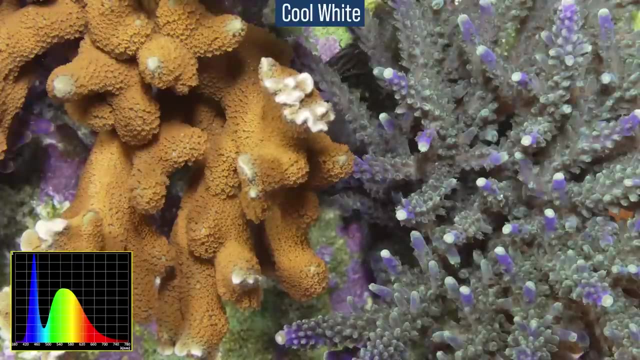 we're back to somewhere around 75 percent fluorescence and we're getting all the orange fluorescence as well. Next we take a deeper look at the other end of blue and how light blue affects fluorescence, which is historically underappreciated in the spectrum offerings Under cool white light. the first coral is brownish orange and the other a muddy. 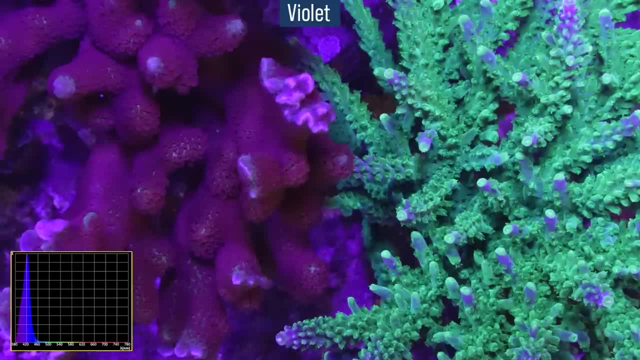 green with purple tips. Under violet light, the coral on the left is a muddy purple brown and on the right the coral is now taking in that violet light and re-emitting it back out as a teal green that just pops, Switching to indigo blue. some of the orange starts to come. 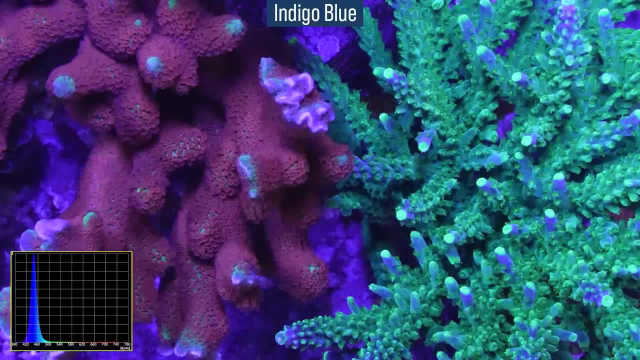 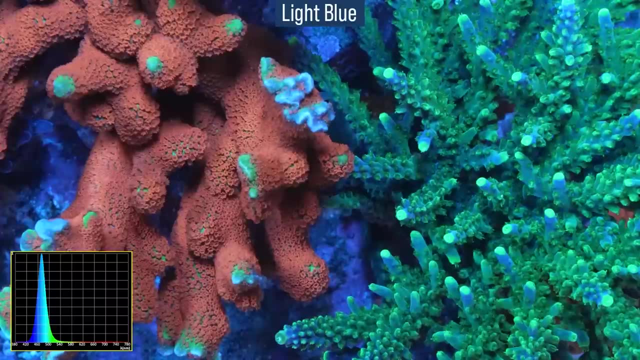 out and there's still a lot of green fluorescence, but just a little bit dimmer Under light blue. that's where the wavelength is. that's popping that orange fluorescence but also highlighting the green fluorescence almost as well as the violet did. Looking at the narrow indigo, 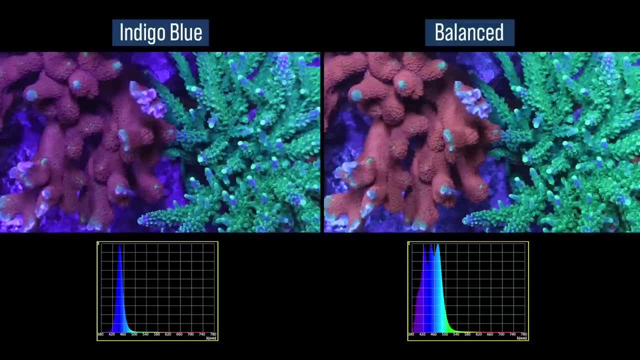 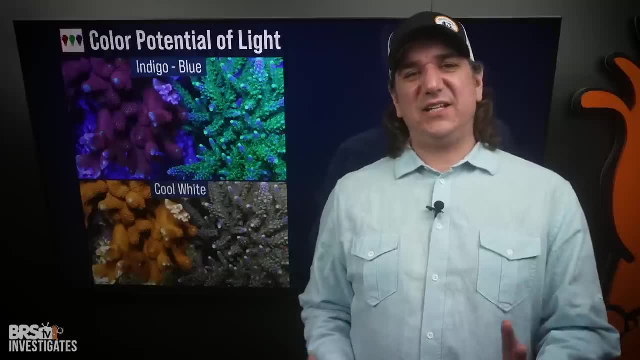 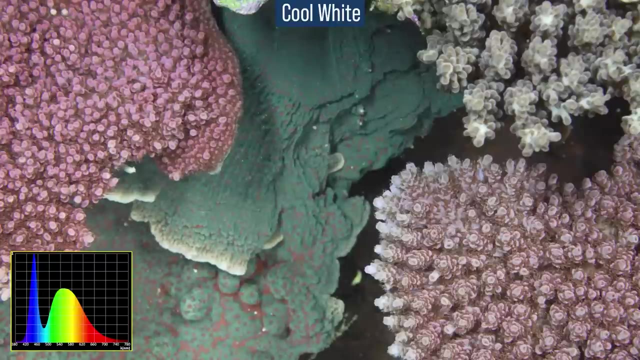 blue, next to the combination of all three- violet, indigo blue and light blue- balanced, the contrast is stark and the oranges are just way brighter. Next set, we selected to highlight what I would call an HDR effect, or high dynamic range of color produced Under cool white light. we see some reds. 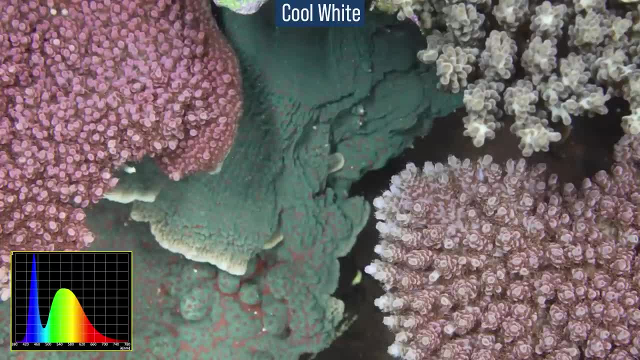 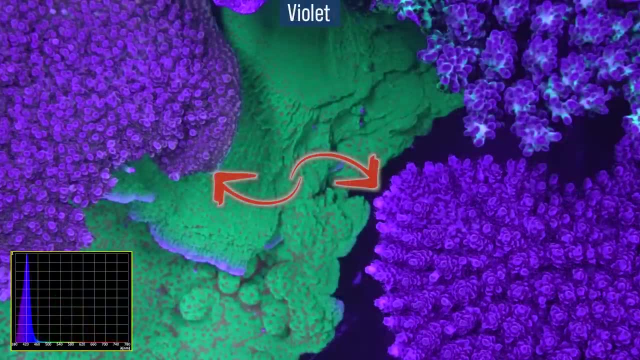 greens, pinks, oranges and yellows. Under cool white light we see some reds, greens, pinks, oranges and teal colors, A bit washed out, but they're all there Under violet light. unlike the previous example, two of these corals actually have very little fluorescence under that violet light. 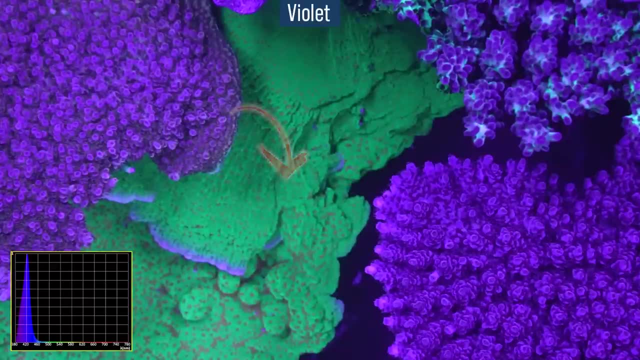 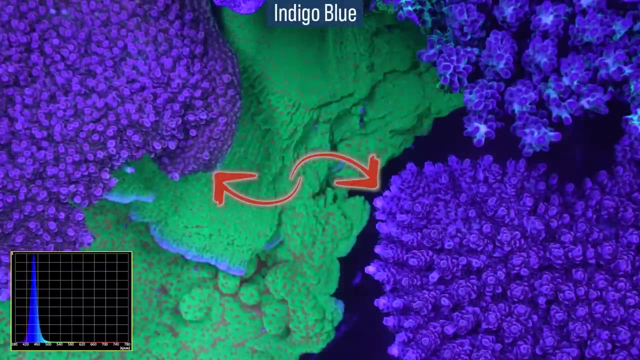 However, the plate is obviously green with orange polyps and in the corner we see some teal fluorescence, which is really cool. Under indigo blue the color shifts to that purpley blue on the left and right, but very little fluorescence. We lose most of that fluorescence. 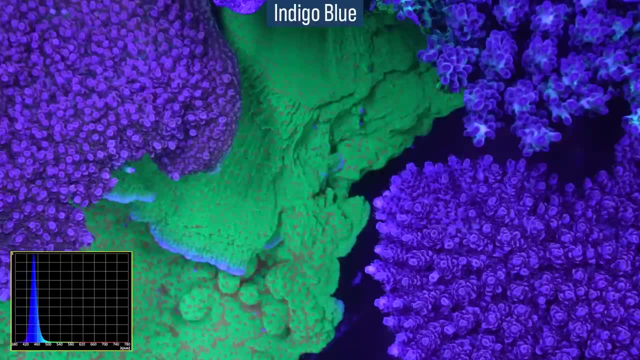 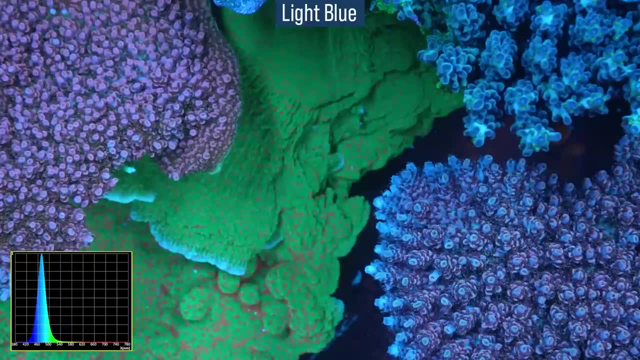 in the corner, but the plating polyps begin to shift to orange Under light blue light. overall that green plate has not changed much under any of these spectrums, but the orange polyps start to glow. You can also see examples of the red fluorescence now as well, Those two corals. 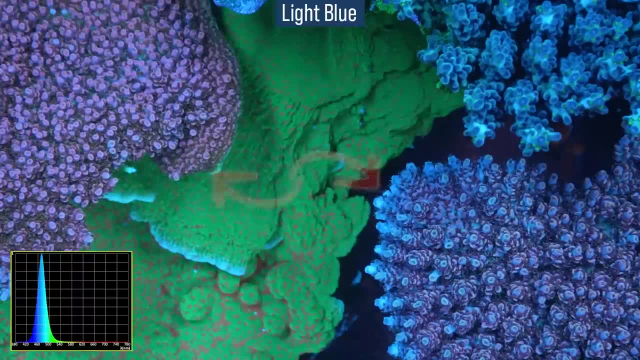 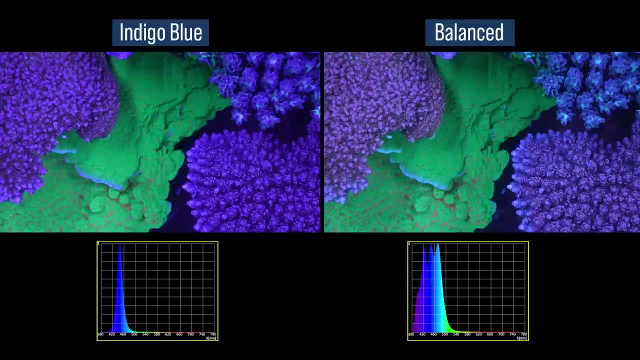 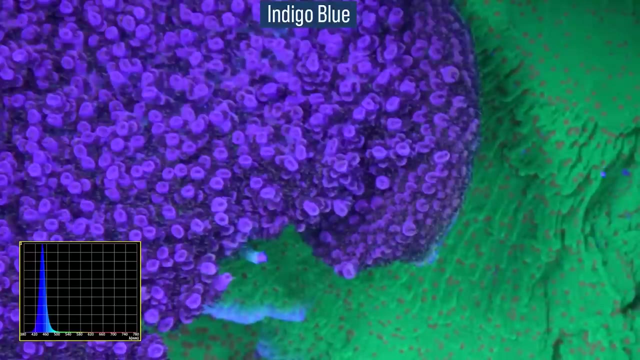 that only had blue pigments before now have very distinct red and pink polyps. When we combine all those spectrums together you see that high dynamic range of color representation. The thin indigo blue peak is kind of one note: green and blue. Looking closer there just isn't a lot of contrasting. 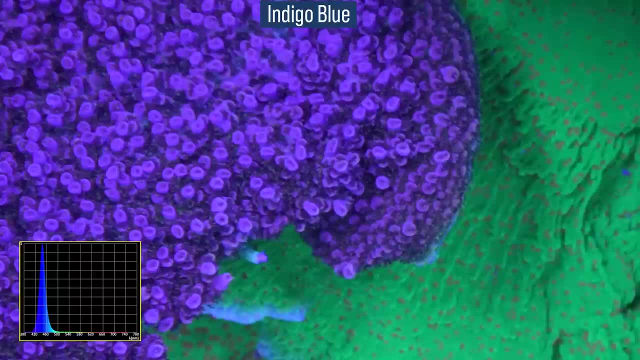 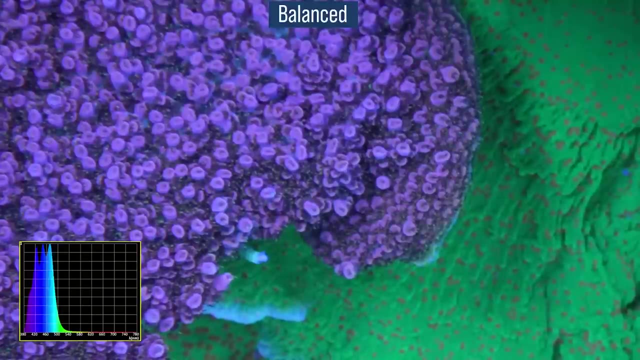 colors and contrasting colors are not the same as the color of the orange polyp. The color of the orange polyp, in contrast, is what makes most of it visually interesting or impressive. However, that wider blue band of mixed violet, indigo blue and light blue produces a wide range of colors and 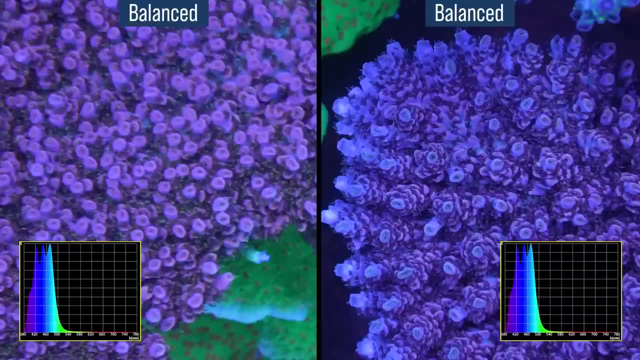 fluorescence. Looking closer, shades of blue intermingling with reds and purples and pinks. In the other case, almost completely, reds and purples and the pinks are dominant with a blue background, And now one is completely glowing, almost like these are different corals, but 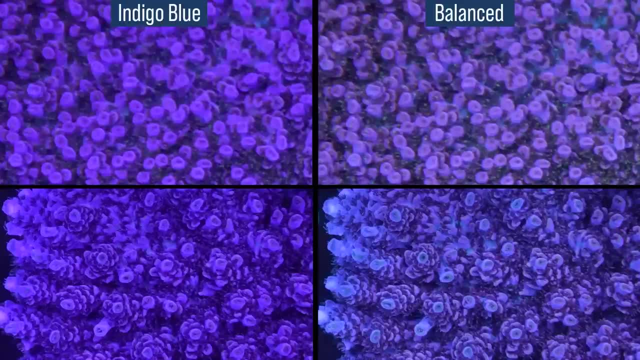 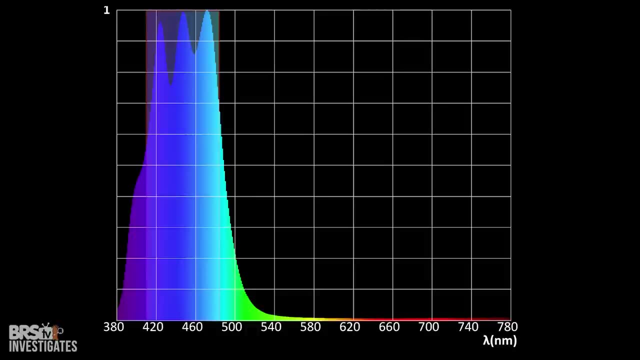 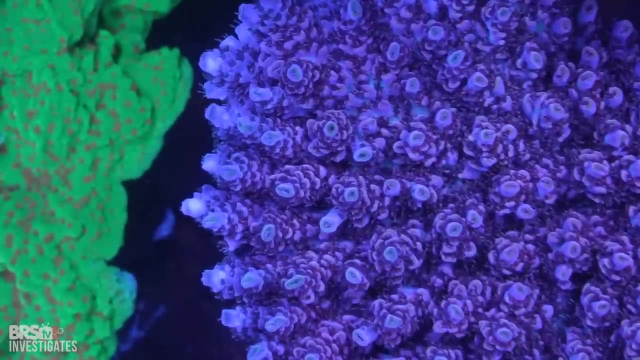 they're not. The only thing that's changed is how we highlight them. So what have we learned? First, that wide blue spectrum we outlined in last week's episode that is optimized for chlorophyll A, C2, and carotenoids is the same wide blue spectrum that highlights corals: natural fluorescence. 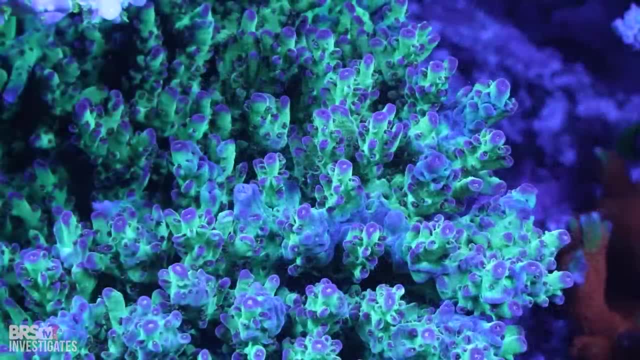 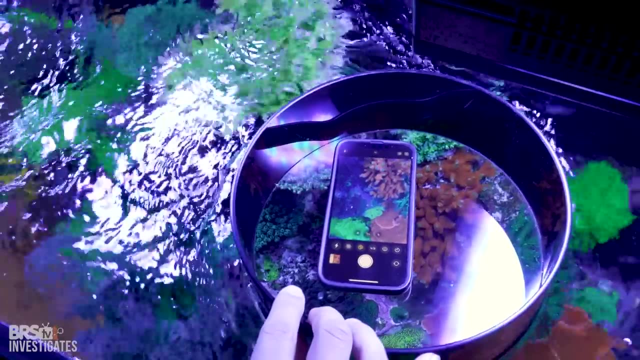 and creates that dynamic range of color depth in all of our corals. What's right for the coral is also right for us. Second, if you shoot your tank with your phone, pick up a look down box like this: If you shoot with a DSLR, get a lens tube like the one from Building Obsession or Advanced. 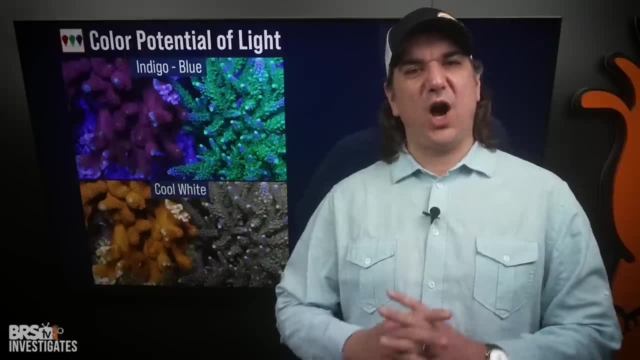 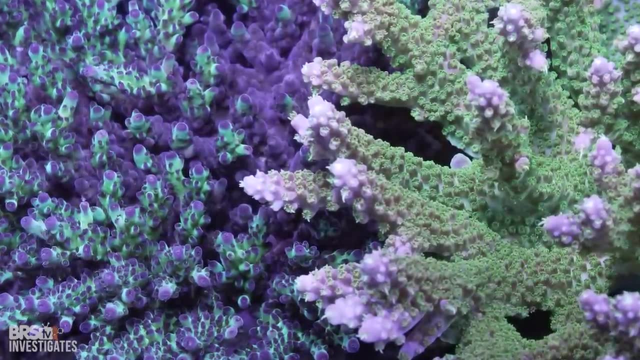 Marine. All of these shots that we took today had zero color correction in editing. You'll be shocked how much better your corals look from the top and how much better you can capture the natural fluorescence with your phone, with no fancy lenses or corrections. Third, why no ultraviolet? 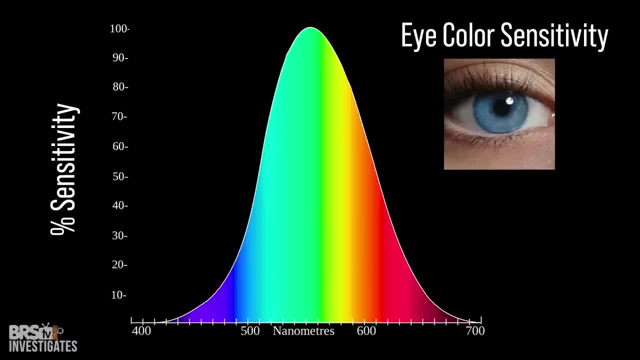 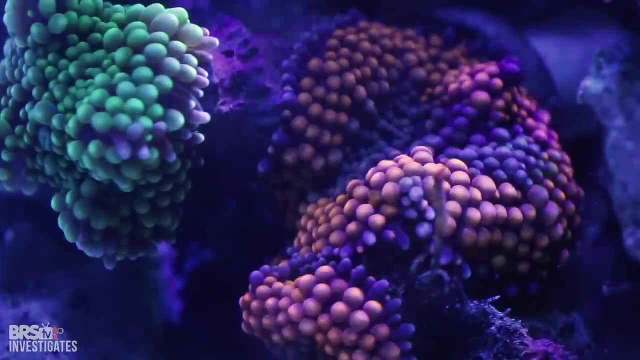 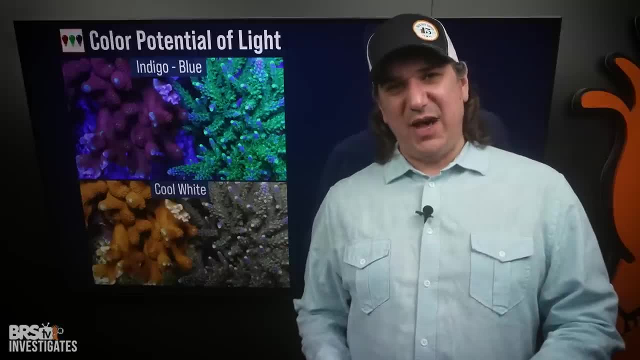 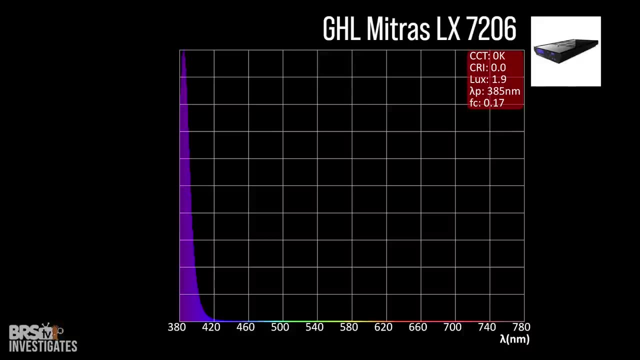 You can see UVA when it's the only channel on. You can see UVA when it's the only channel on Which easily overpower it. Note that I am not talking about the channels that are labeled by the manufacturer as UV, which is often just marketing for deep violet, but actual 380 to 400 light, which most lights have. 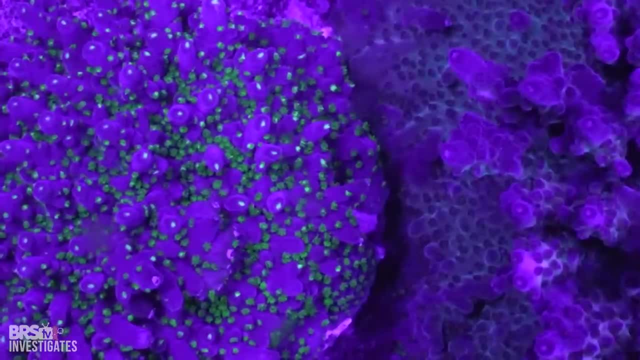 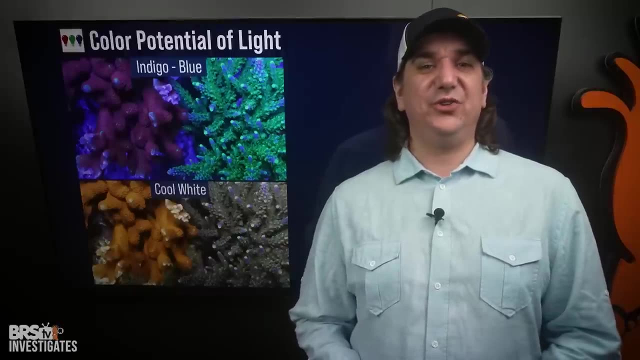 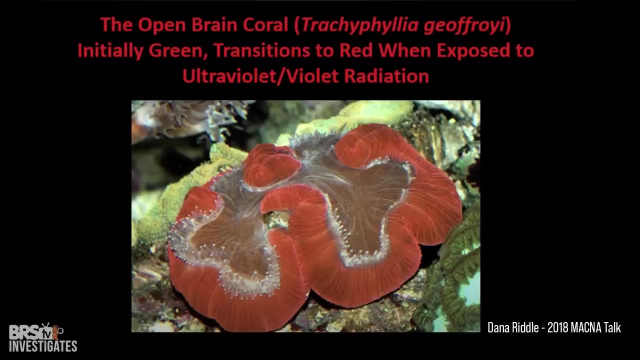 very little of The potential benefits of near UV is more of a biology question than a color question. There's one caveat to that. Both UV and violet light can cause the coral to change the fluorescent pigment content within the coral often noted, with a transition between green to red, depending. 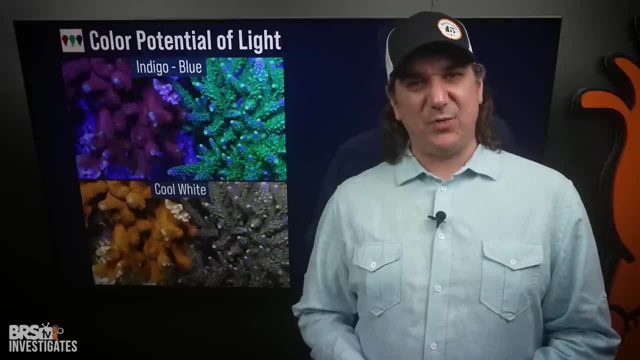 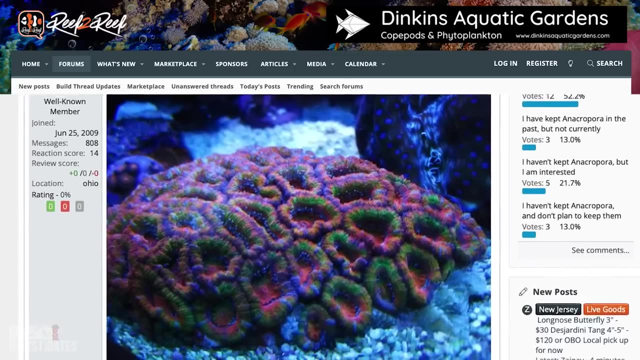 on the amount of UV, So some aspects of the light spectrum can actually change the actual color of the coral over time, not just highlight it differently. However, having your rainbow acans turn all red might not be the desired effect that you were looking for. 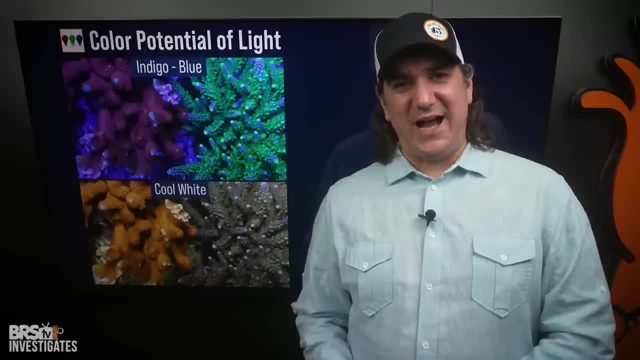 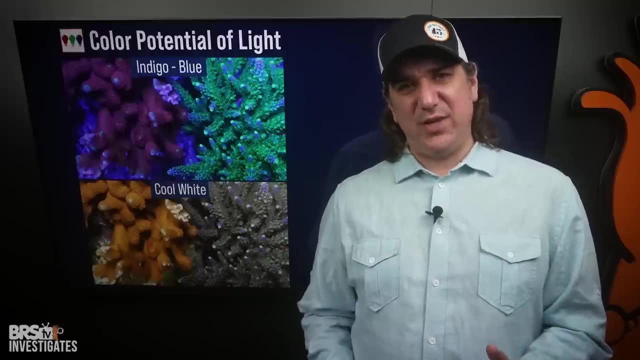 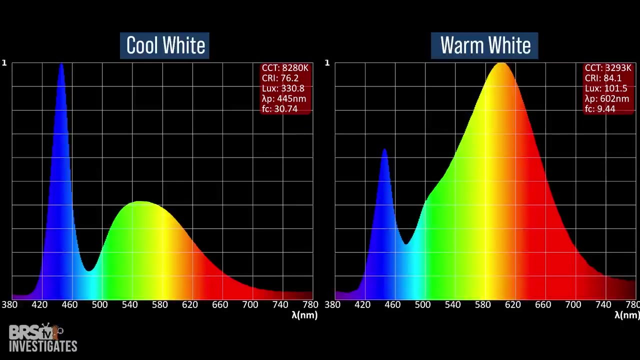 Fourth, why didn't we explore color pigment or white shots? The color is largely just provided with the white channels, which include all the other spectrums, sometimes with the ability to boost red and green. One note here is the difference between warm white and cool white. They often have a similar color offering, with the exception. 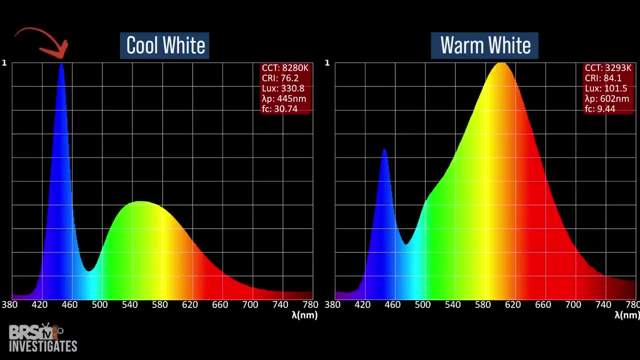 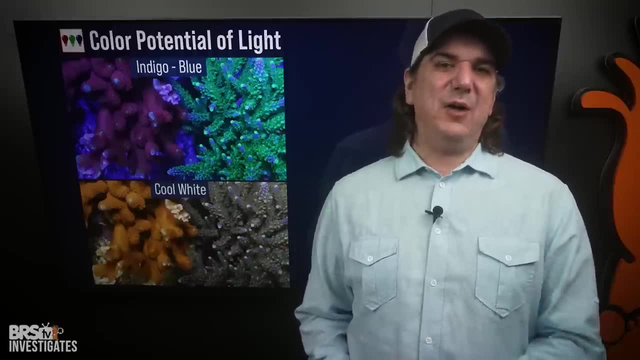 of the cool white having a strong 450 indigo blue peak, Since most reef tank lights actually have plenty of those royal blue LEDs and don't really need more with the whites, I wouldn't be surprised if there continues to be a trend towards using more warm whites over cool whites in the future. 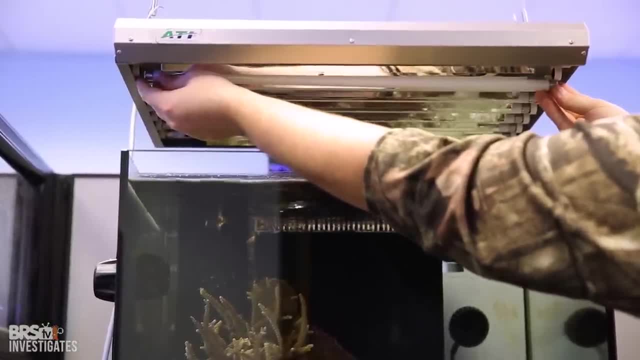 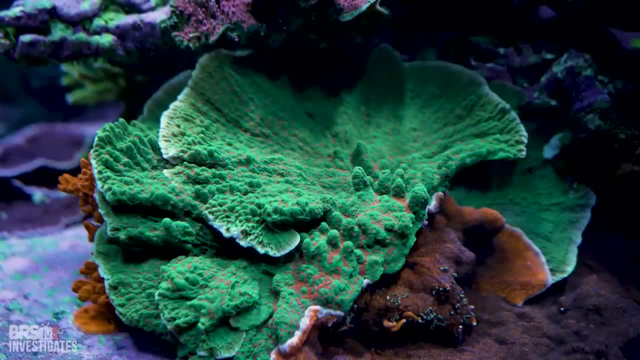 Fifth, there's no right answer to all of this. It's why people have been swapping out halide and T5 bulbs for ages, mixing them with LEDs. I don't think that's the right answer. Every tank will have different corals in it, which are highlighted with a wide array of spectrums. 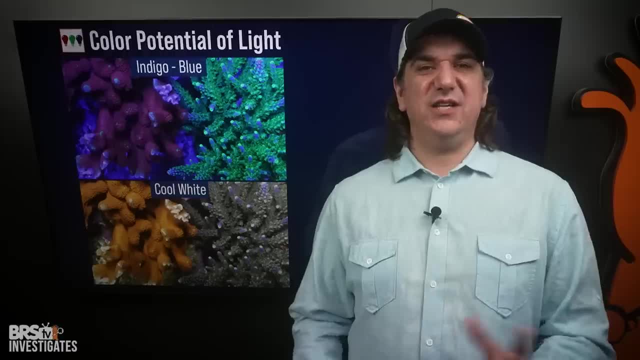 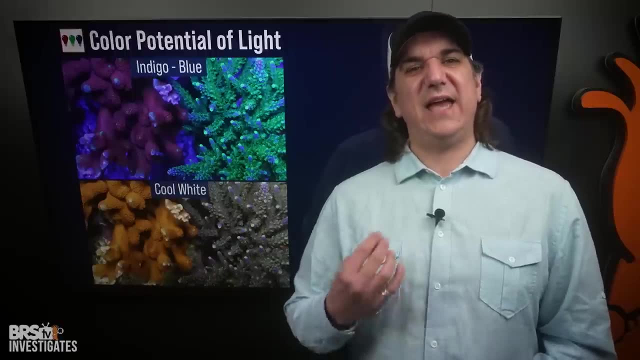 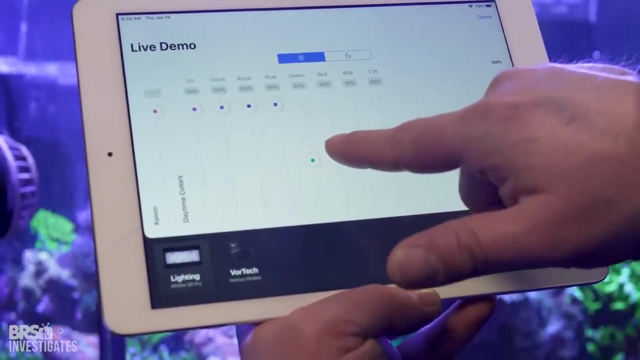 that is blended to highlight them the best. The color is a personal preference, but starting with a wide blue spectrum and then intelligent control over each color peak is the most capable solution. The ability to do that with a finger slide instead of buying and swapping out bulbs, is one of the reasons why reefers have gravitated to LEDs so rapidly. 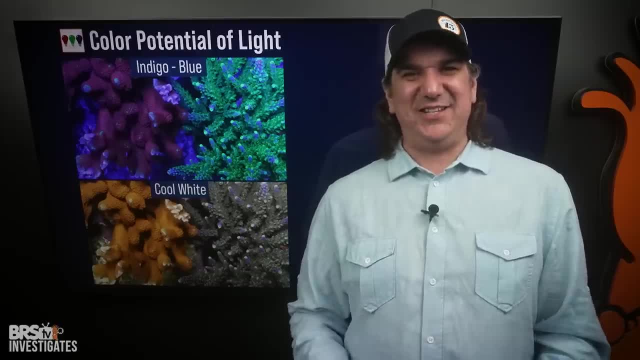 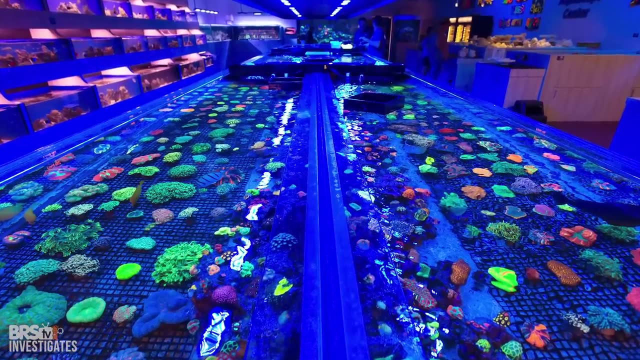 Sixth, the easiest way to get the best fluorescence is to actually take a blue LED light to the store and only buy the ones that glow. Second, aquaculture corals grown under artificial light are much more likely to keep that coloration when they're transitioned to your tank. 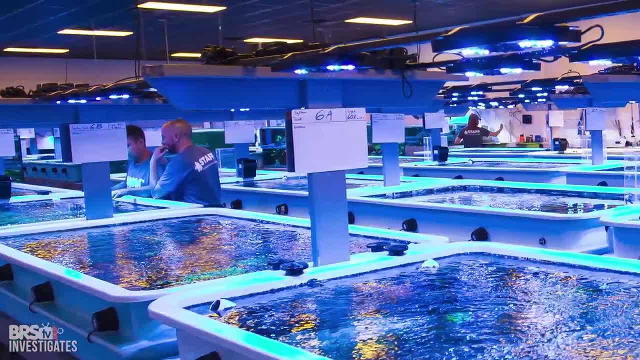 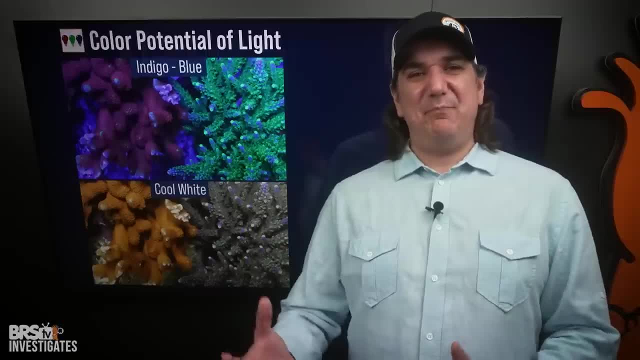 than with wild caught corals. If possible, ask the store what lights they use and their spectrum mix to come close to ensuring that you keep that color that you paid for. Seventh, what is that balance setting that we use to get that blue blend that we use today? 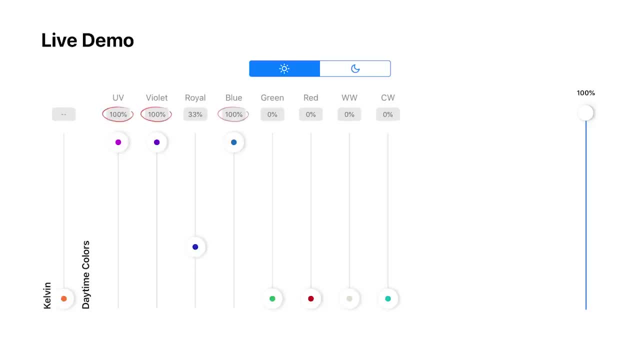 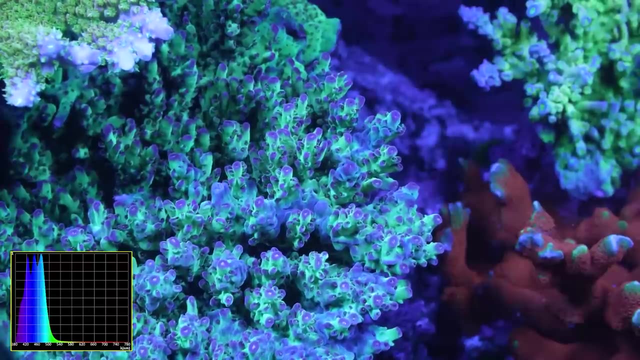 with the radions on the 750?. It was UV, violet and blue all at 100% and royal blue at 33%. This ended up with a fairly balanced blended spectrum which will actually look lighter blue because of the human eye's higher sensitivity to light, blue, light Blending. 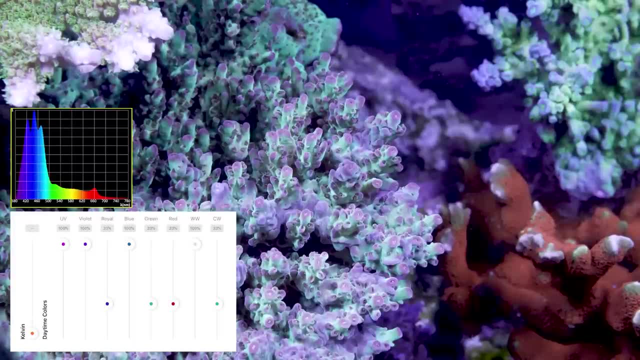 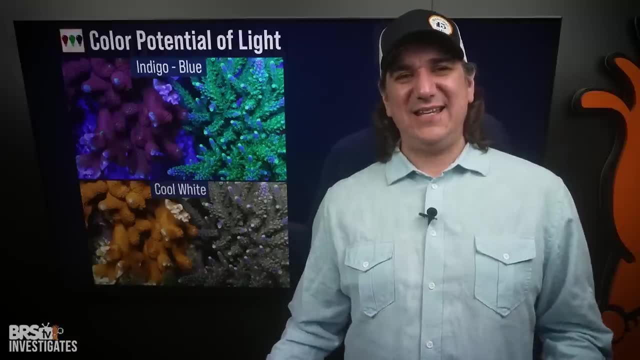 that, with 100% warm white, with 33% red and green, created an overall nice look and a very balanced wide blue band. Eighth, the biggest question of the day: what if my light doesn't have the violet or light blue spectrum? How do I supplement it to get the best fluorescence? Buying new lights is